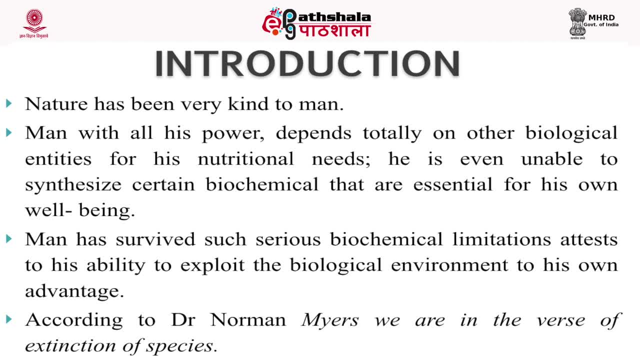 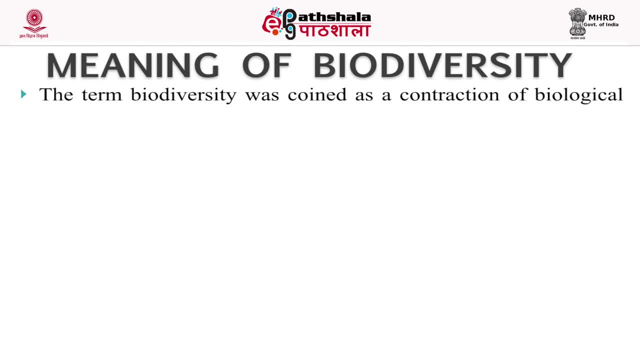 of environment is biological resource, which includes biodiversity. Now I would like to discuss what exactly do we understand by this term biodiversity? The term biodiversity was coined as biological resource. Biological resource is a resource that is used for the survival of life, Both the Carris and the 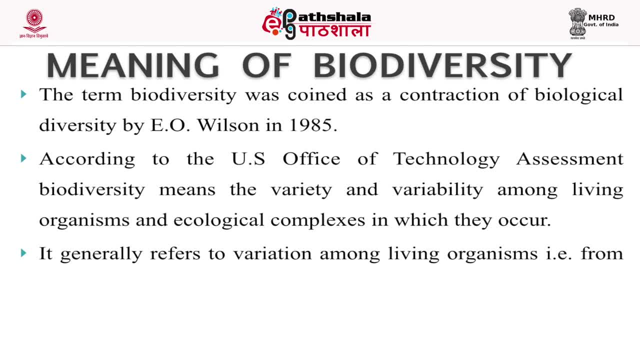 Bream have the following key features: Biodiversity means the diversity and variability among living organisms and ecological complexes in which they occur. It generally refers to variation among living organisms, that is, from the molecular unit to individual organisms and then onto the population, community, ecosystem, landscape, and further also refers to genetic diversity based on how. Ball-S Госüt они. 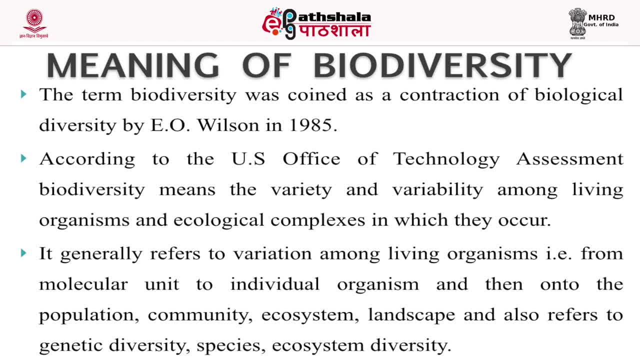 chekn mastね, And it is also referred to some ways as geneticอนюсь CDEZ, or With respect to trace- За biodiversity, species, ecosystem diversity In the widest possible amplitude. biodiversity is taken to be the aggregate of life on earth. I like to repeat here that it is taken to 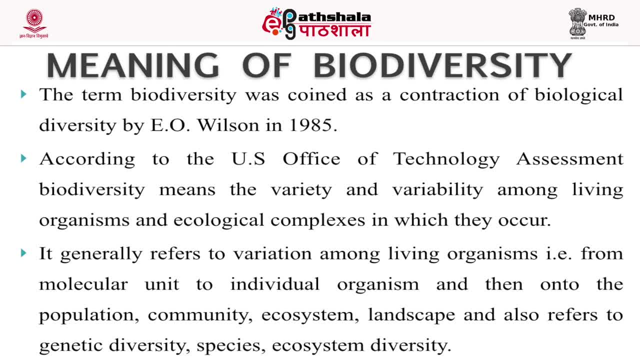 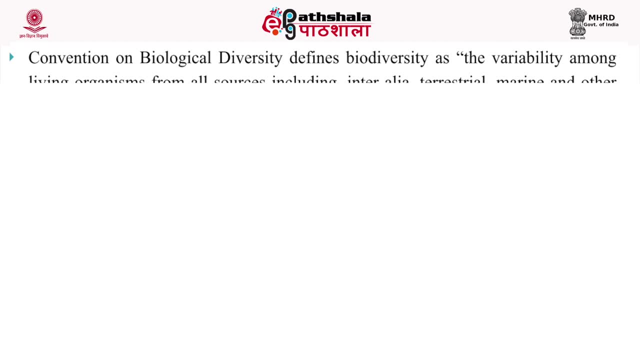 be as an aggregate of life on earth. So therefore it can be concluded here that the total of life form, no matter how big or small it may be, is included within the ambit of biodiversity. Statistice definition on biodiversity defines biodiversity as the variability among living. 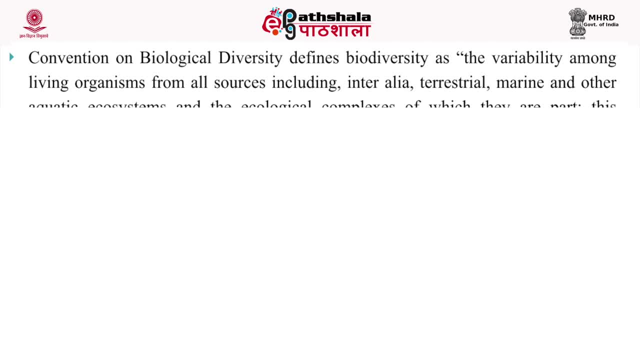 organisms from all sources, including terrestrial, marine and other aquatic ecosystems, and the ecological complexes of which they are a part off, And this includes diversity within species, between species and of ecosystems. The definition of biodiversity under the Biological Diversity Act is the variability among living 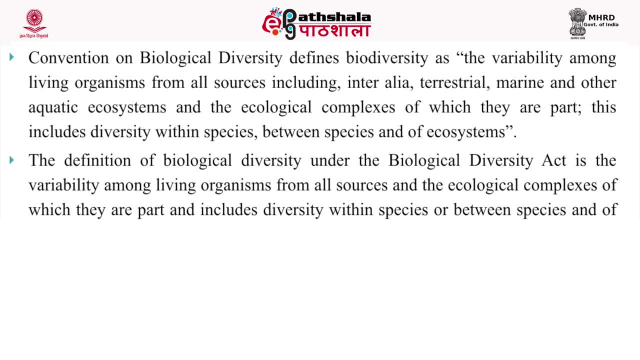 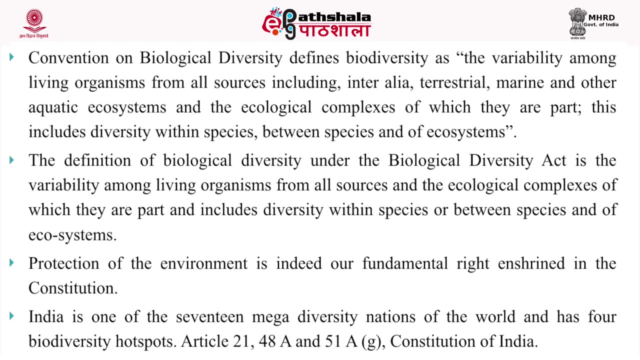 organisms from all sources and the ecological complexes of which they are a part of, and include diversity within species or between species, and of ecosystems. Protection of environment is indeed our fundamental right, as enshrined in the Indian constitution. India is one of the 17 mega diversity nations of the world. 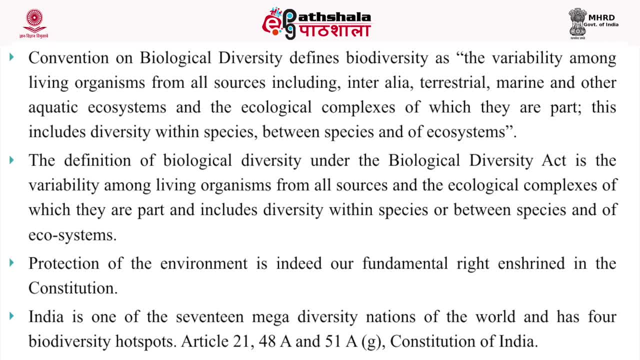 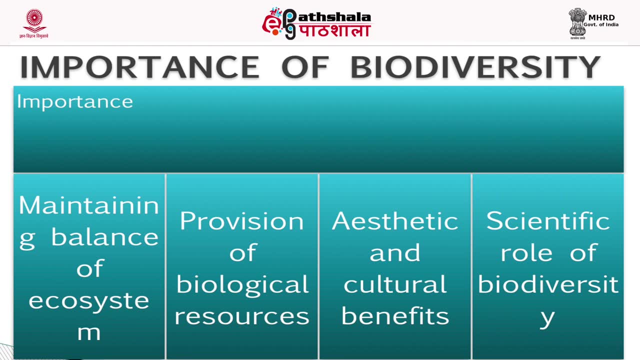 and has four biodiversity hotspots. India contains 668 protected areas, comprising of wildlife sanctuaries, national parks, tiger reserves, elephant reserves, community reserves and conservation reserves. India is recognized as one of the eighth pavilion centers of origin and diversity of crop plants and possesses more than 300 wild ancestors and close relatives of. 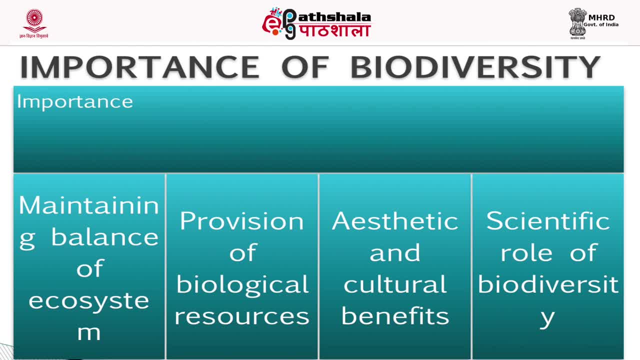 cultivated plants which are still evolving under the natural. It has also taken to be as a vast repository of traditional knowledge associated with biological resources. Now the second point of my discussion is: what is the basic importance of biodiversity, and when we try to interpret this biodiversity, or the importance of biodiversity, then it can. 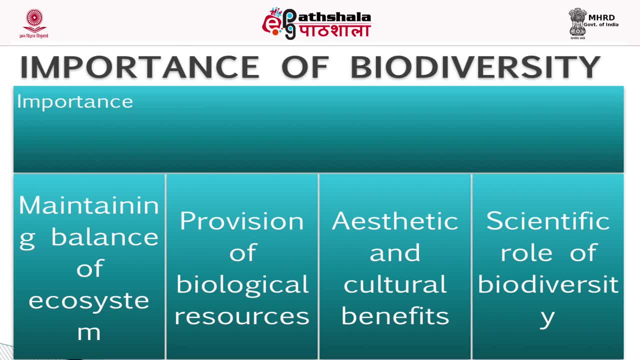 be summarized as under: first, biodiversity helps in maintaining balance of ecosystem. I would like to explain here that one of the essentials of biodiversity is that it helps in maintaining balance of ecosystem, and it does that by various ways, like constantly maintaining the balance of climate and atmosphere. It helps in not just storing the essential nutrients. 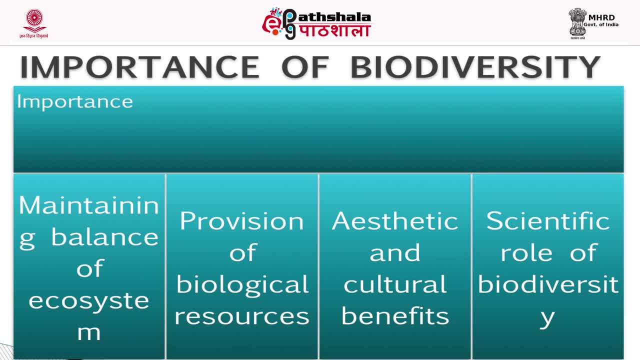 present, but also makes them reusable. It helps in curbing and preventing the pollution, which can be taken to be as the main cause for the loss of biodiversity. It preserves the water channels and prevents the soil erosion, which can again be taken to be as a cause of loss. 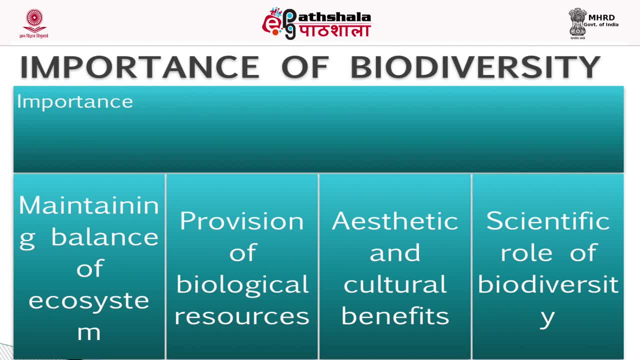 of biodiversity. Second, sources of biological diversity. Biodiversity is also a major source of providing biological resources, which can be helpful in many ways, like providing of drugs to cure and prevent various diseases, acts as a source of nutrition for both human beings and animals, and acts 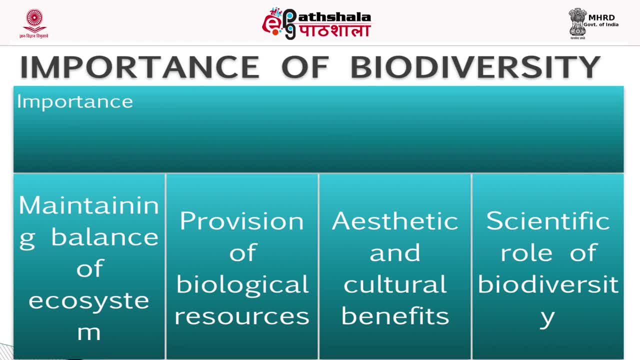 as a breeding ground for the life on earth. Third, aesthetic value and traditional benefits. Biodiversity has great aesthetic value and acts as a source of income as well. One of the examples for this can be the parks, the sanctuaries, the reserves which are established. 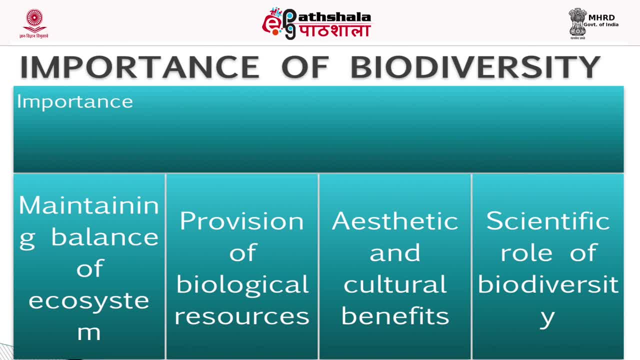 for the viewing of people of various flora and fauna. Example of aesthetic value includes ecotourism, bird watching, wildlife gardening, etc. Therefore, it can be said that it helps in increasing the ecotourism because it acts as a source of entertainment, knowledge and 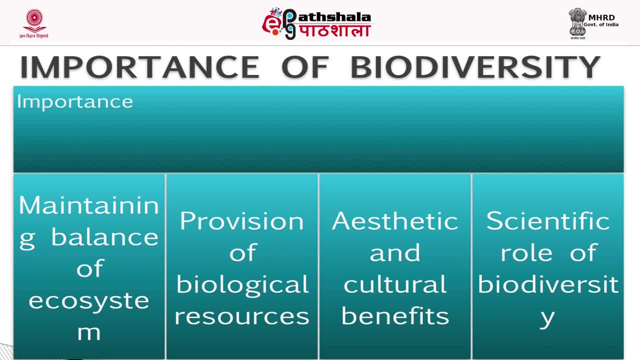 information. Also, they have traditional value because in India it is seen that some of the plants and animals are worshipped, like people, tree tulsi, and animals like cows and snakes, which are taken to be animals which are to be worshipped. Fourth, scientific role of biodiversity, One of the major role which biodiversity can play. 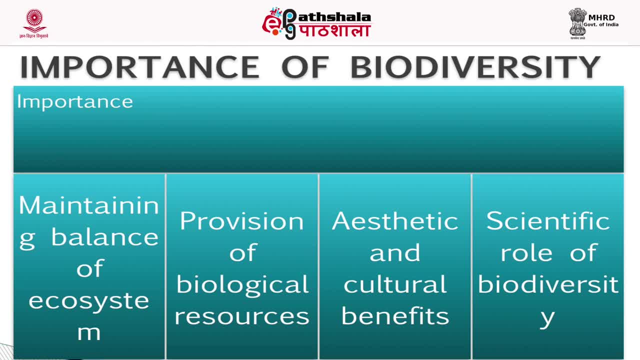 is through the scientists. The scientists, by studying and experimenting on these species, can come to the conclusion that how the life actually started and to know what levels these species can go to sustain themselves. Also, further, as we all know that biodiversity today is at great risk because both natural 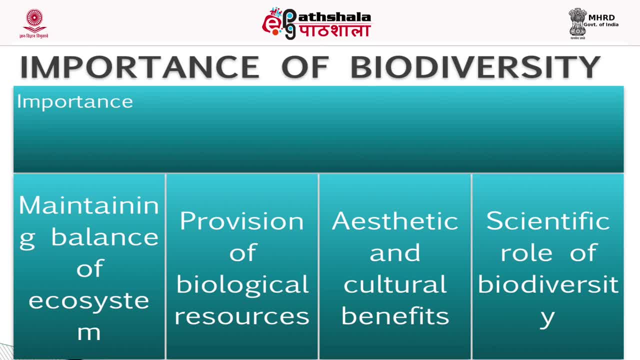 and manmade reasons, and every possible effort is made at national and international level to protect and conserve biodiversity. So, therefore, these scientists, by studying these species, can come to the conclusion of the steps taken for the conservation of biodiversity. The next part that we would be discussing is the types of biodiversity. 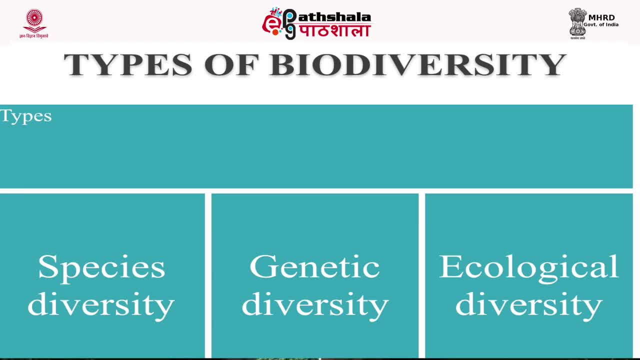 We have already evaluated the importance of biodiversity. We have evaluated what exactly do we understand by the term biodiversity? The next important question is that we need to answer: what are the different types of diversities? and they are basically three types of biodiversities or diversities. 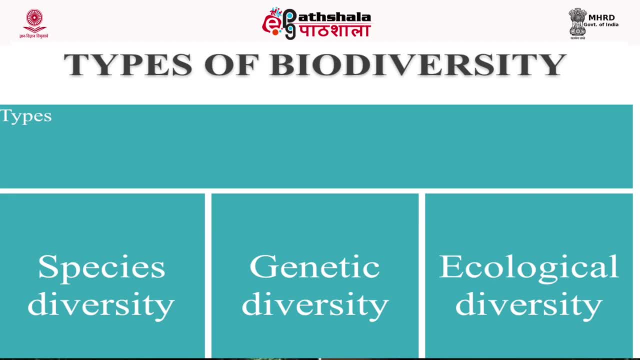 First, genetic diversity. Genetic diversity is generally said that genes of a person pass from one generation to another, and there might be times when there is variation in the genes that pass from one generation to the other. The connection that is drawn between two individuals is through the similarity in their genes. The more the similarity between the 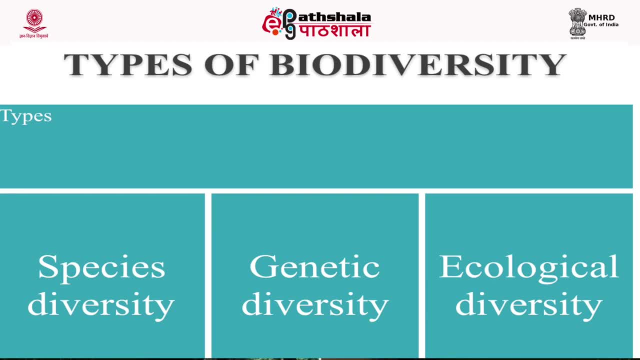 genes of two individuals, the more closely related they are towards each other. The second type of biodiversity or diversity is species diversity. As we all have already discussed genetic diversity, so the next important type of diversity is species diversity, because genes make species Species. diversity means and includes the living creatures present in the ecosystem. 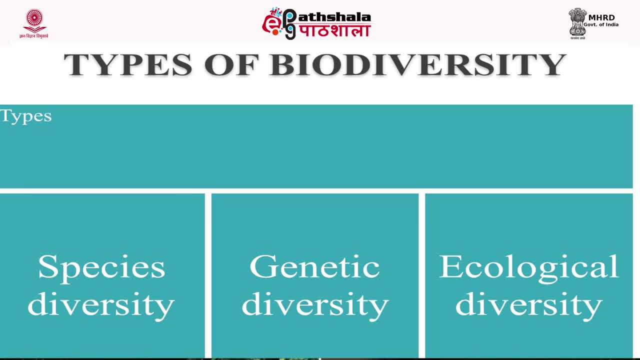 and this includes both flora and fauna. There is always an interaction that is taking place between various types of species present in the ecosystem. Species belonging to the same group can be taken to a group in which reproduction can take place through breeding. The third type of diversity is ecological diversity. Ecosystem generally means the blend. 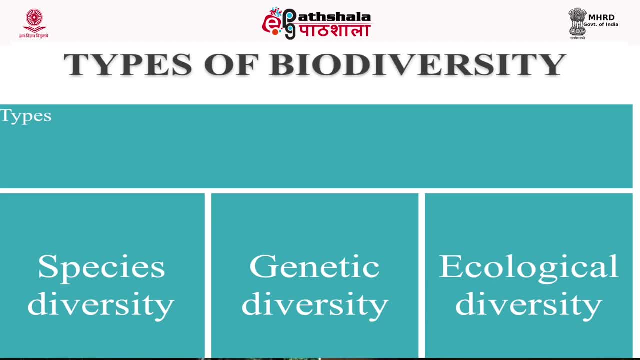 or amalgamation- I repeat, blend or amalgamation- of different living creatures in the physical environment and the interaction between both of them. Basically, all the living space for all species on earth is provided by ecosystems in form of different habitations. The beauty. 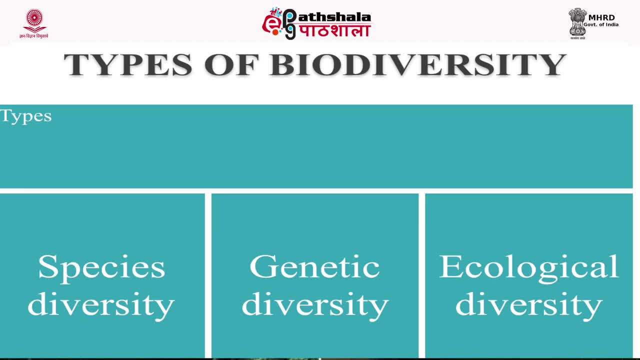 of this ecosystem is. it plays different roles and provides different types of habitations to different types of living creatures, depending on their needs. This is all fulfilled by the diverse types of biodiversity we have that accommodates all types of flora and fauna and gives them a living space. As I have already discussed the fact that the ecosystem is diverse, 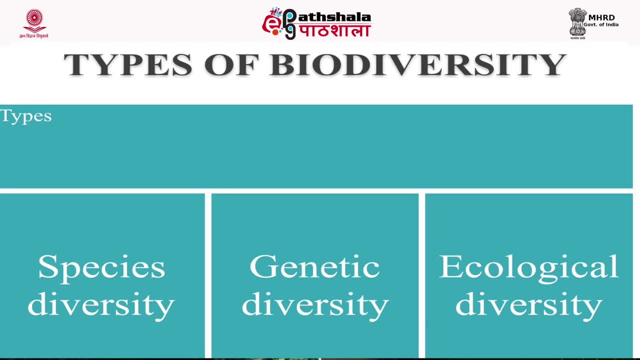 in nature and accommodates all types of living beings. the irony of the situation is that this system is never stable and it keeps on changing, and sometimes this change is for good, but at times it may also not be for good, which might lead to extinction of various flora. 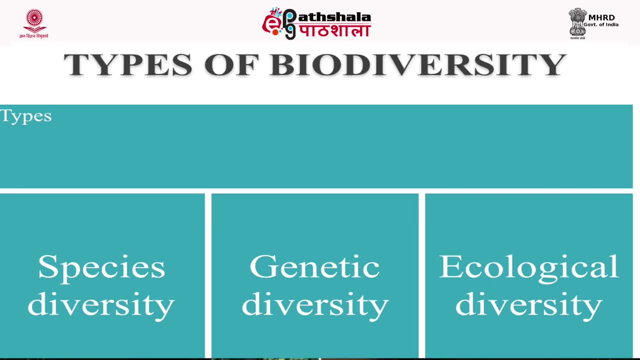 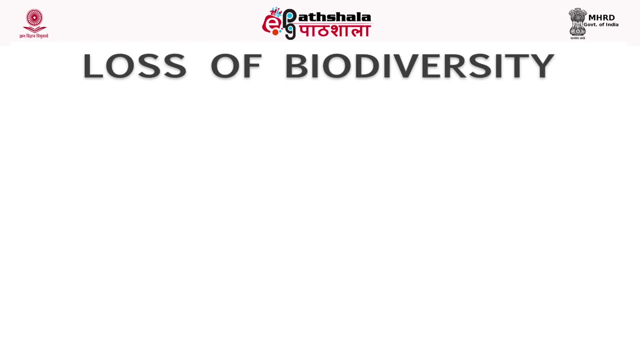 and fauna, And this extinction is the major cause of concern for both national and international community. So, therefore, preservation of ecosystem is necessary, so that interaction between both physical and living components can take place without any adverse effect on biodiversity. Now the next part that we would be discussing is loss of biodiversity. Now, after discussing 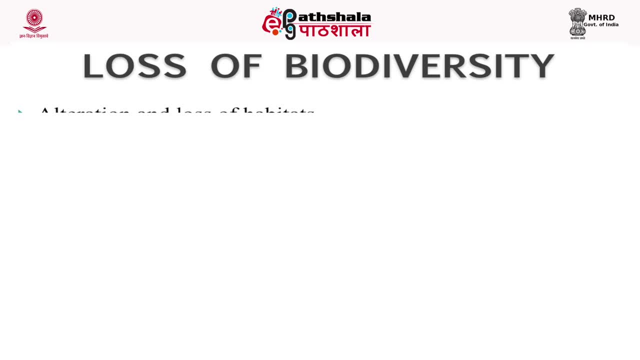 the importance of biodiversity, the types of biodiversity and the definition of biodiversity. the next important question is: what are the various reasons for the loss of biodiversity? Unquestionably, the most important concern of the world today is the loss that is occurring with respect to biodiversity, and that, too, in almost the whole wide world, This depletion. 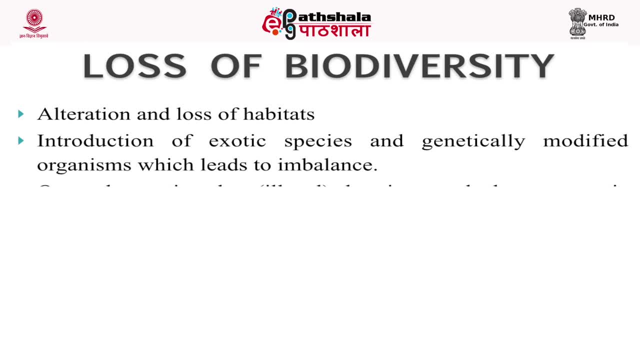 that is taking place is taking place as a very fast pace because the loss is taking place rapidly. therefore, it is a grave matter of concern for both national as well as international community. So let us start. Some of the reasons for the loss of biodiversity are, first, destruction and variation of ecosystem. 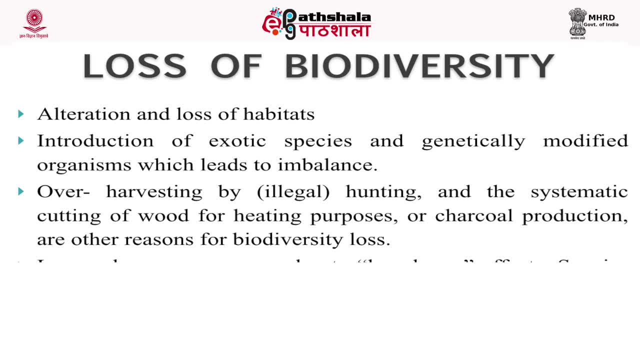 One of the major reasons in the damage to the biodiversity is destruction and variation in the ecosystem. There is always a set pattern in the ecosystem where exists or where the existence of living organisms takes place. and even if there is a change in the ecosystem, the change is of such a nature that the environment is favorable for the birth and the growth of. 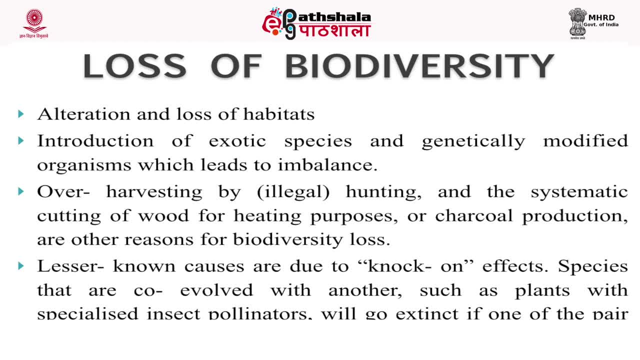 the living organisms, But because of the fact that the agricultural land is decreasing, cities and buildings are increasing. it is causing destruction to the ecosystem, which in turn affects the biodiversity and damages it Also further. there is a loss of the natural habitat of flora and fauna and suitable conditions. 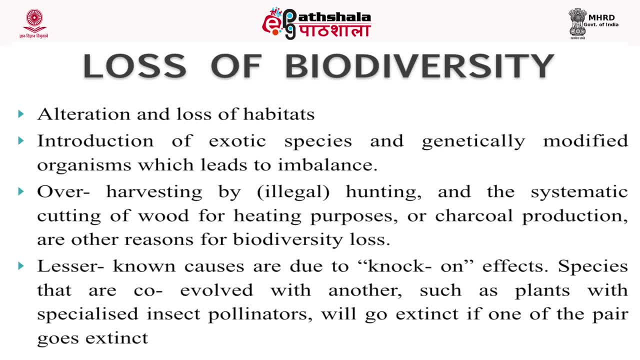 of growth are not being given to them, because of which there is a loss of biodiversity. The second point is various new and exhausted species being added to the ecosystem, in addition to genetically modified species. This is the reason why we are in such a state of prematurely. 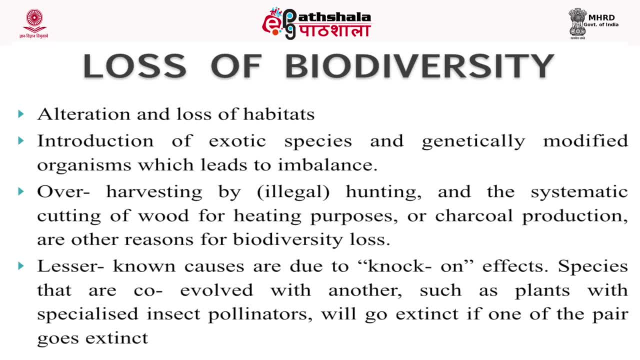 genetically modified organisms. One of the major threat to biodiversity is that of new species being added to the ecosystem when at times, or which at times can become dominant to the species already present, and creating an imbalance in the ecosystem. Further, because of the development of biotechnology, we are seeing the growth of genetically modified 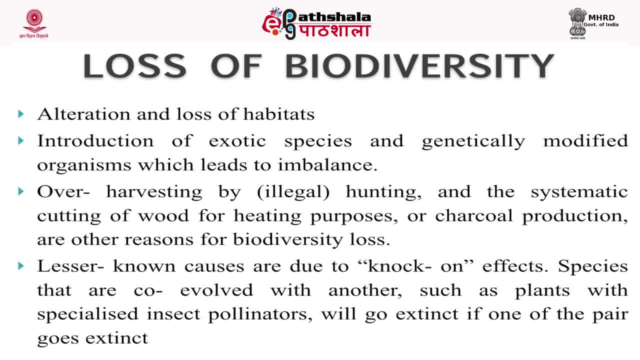 organisms and plants which, at times, can be resistant to various animals and insects of that area, again creating an imbalance. Third, threatening the forests by cutting of trees, because of which the forests, which act as a natural habitat for various plants and animals, are decreasing, which is in turn also leading to soil erosion, And this soil erosion is: 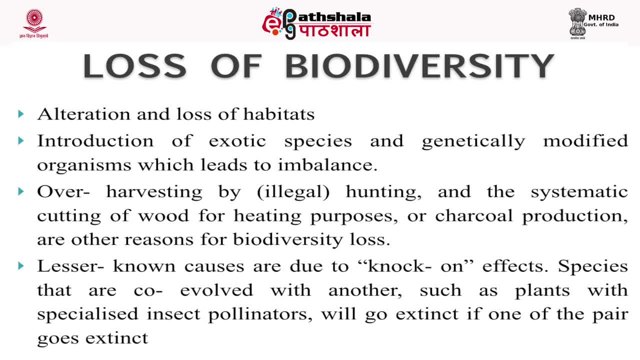 affecting the fertility of land, which in turn acts as a major concern for the loss of biodiversity. There are some species which are bound to exist in a certain particular habitat within the existence of certain other species, and in this case, if one of the species is affected, there would be the loss to the other. 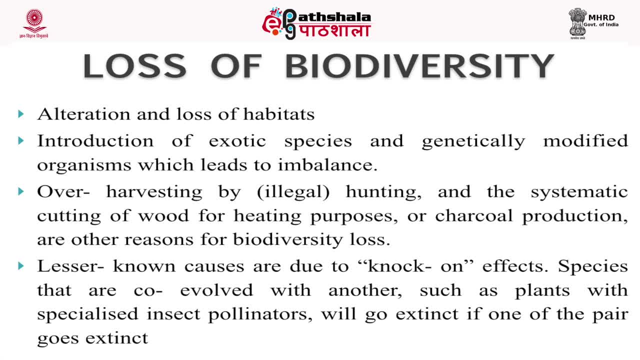 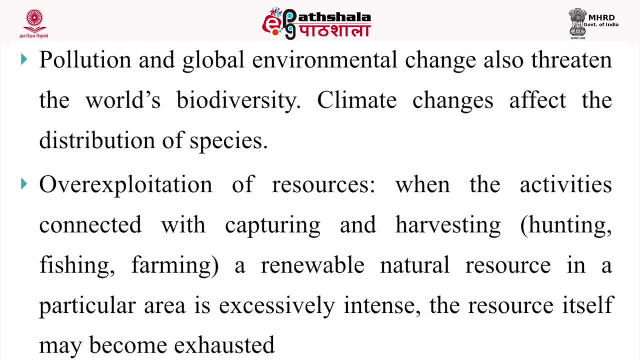 This would also mean that the food chain would be destroyed. This is known by the name of knockout effects. Pollution and global environment can also threaten the world's biodiversity. Climate change also acts sorry as a distribution of species and helps or affects the biodiversity negatively in the depletion of the species. 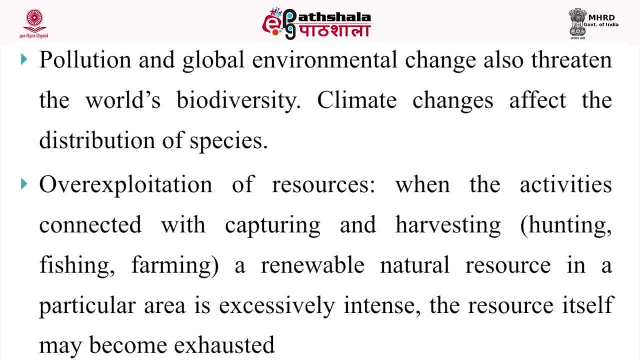 Overexploitation of resources. Overexploitation is generally taken to be opposite of sustainable use. When we go to the extent of exploiting the resources which are limited in nature without keeping the future needs into prospective, this would in turn lead to the loss of biodiversity. 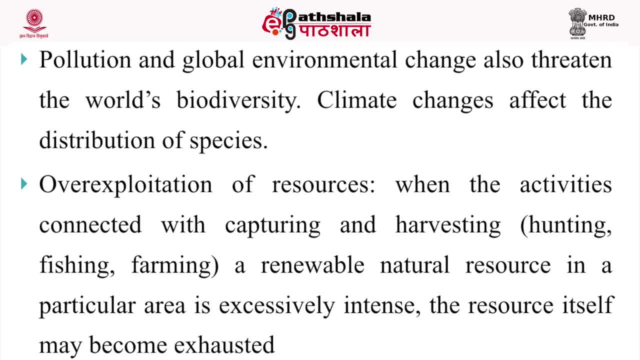 So, keeping the above points in mind, every possible effort should be made by human being that the loss to the biodiversity should not take place, and the preservation and conservation of it should be taken to be as a concern of not just the few but all. 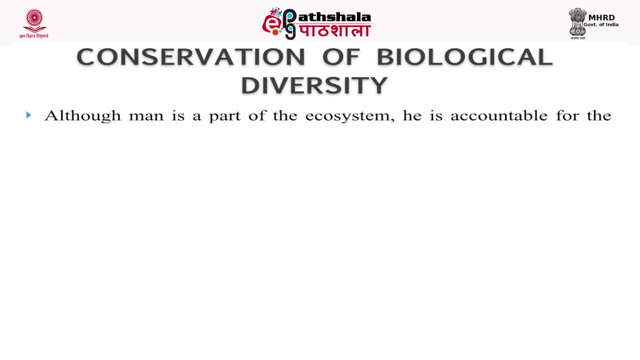 Now the next point is conservation of biodiversity. Although man is a part of ecosystem, he is accountable for the degradation and depletion of the biodiversity. Though, as compared to the flora and fauna, the number of human beings are less the damage they have done to the 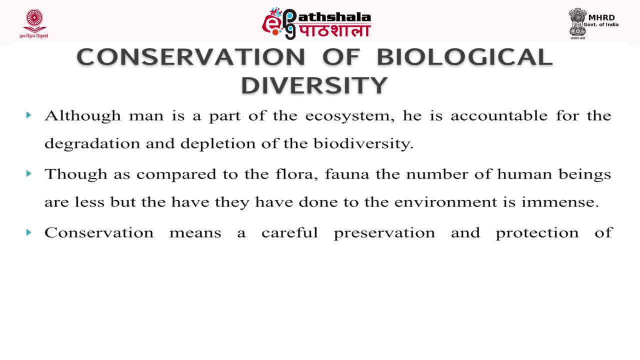 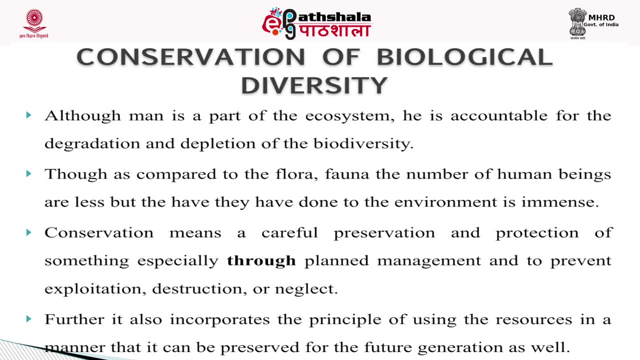 environment is immense. Conservation means a careful safeguarding and gardening or guarding of something, especially through plant management and to prevent abuse, damage or neglect. Further, it also incorporates the principle of using the resources in a manner that it can be preserved for the future generation as well, which is also known by the name of the concept of sustainable. 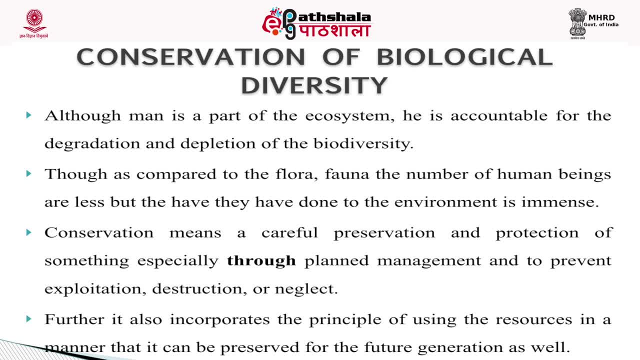 development. It is expected that, with the increasing awareness towards the values and importance of biodiversity and stringent measures, we shall be able to protect our biodiversity. We need the need to conserve biodiversity, keeping in view the direct use values, indirect use values and intrinsic values of biodiversity. In fact, the very existence of human species and sustainable 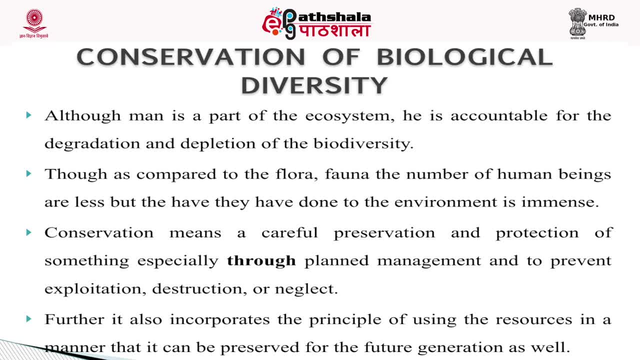 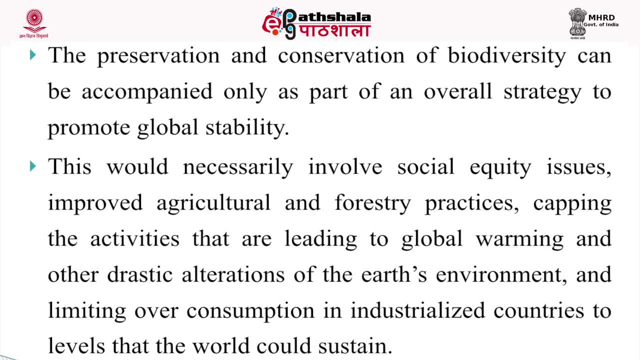 development depends on biodiversity conservation, Both institute and ex-suite. conservation has to be a part of the cultural tradition in India. The preservation and conservation of biodiversity can be accompanied only as a part of an overlapped strategy to promote global stability. It is a need of the art that all the 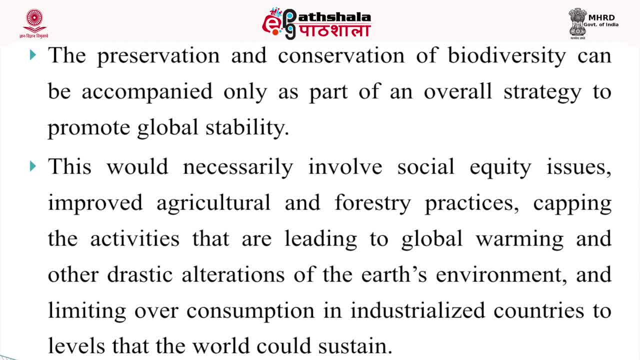 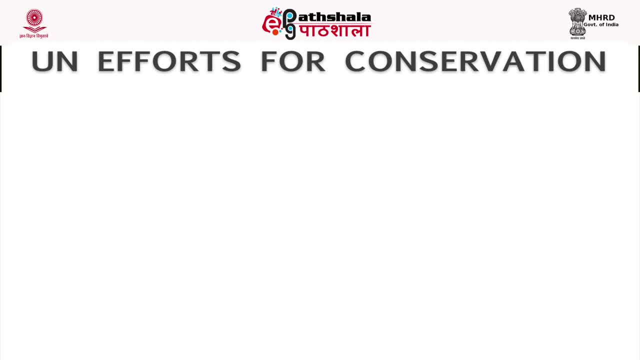 countries come together to take concrete steps for the conservation of biodiversity. Some of the techniques we are going to discuss today include collaboration with the United Nations for conservation of biodiversity. Conservation is closely linked with human activities that reap the benefit of human beings by harvesting, consuming and utilizing. 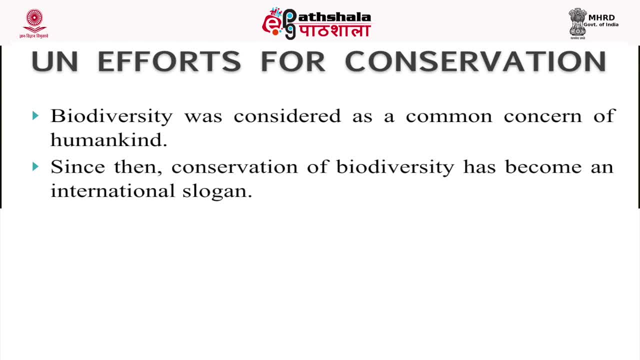 the resources. However, in absence of knowledge on the importance of conservation of these resources in a sustainable manner, people tend to consume excessively, leading to depletion and the loss of biodiversity. There are also the responsibility for bibliques and other Biodiversity was considered and is considered as a common concern of humankind. 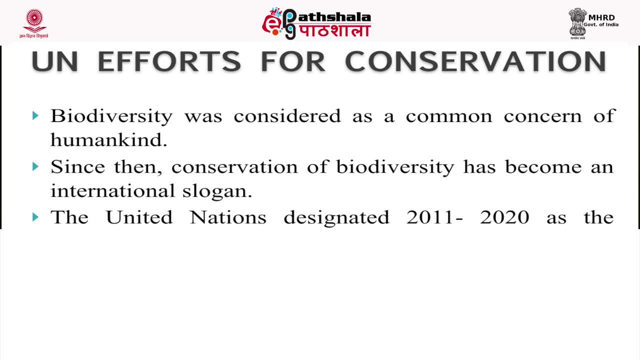 Since then, conservation of biodiversity has become an international slogan. 2011-2020 has been designated as the United Nations Decade on Biodiversity, wherein different steps would be taken by the United Nations first and all the member countries for the preservation and protection of biodiversity. 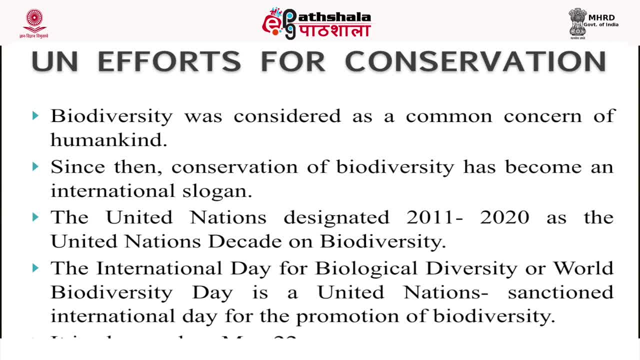 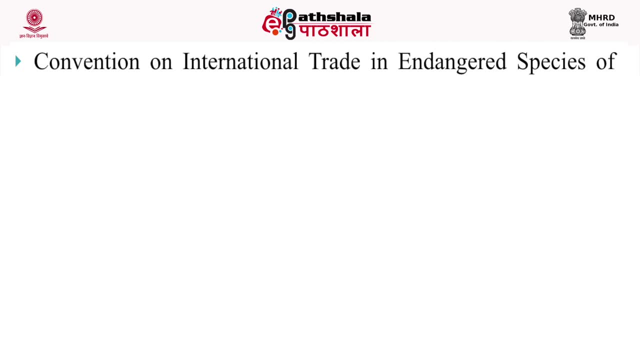 Further. in light of the above statement, May 22nd is celebrated as International Day for Biological Diversity or World Biodiversity Day. The first step taken by the United Nations worth acknowledging for the conservation of biodiversity was making the Convention on International Trade in Endangered Species of Wild Fauna and Flora. 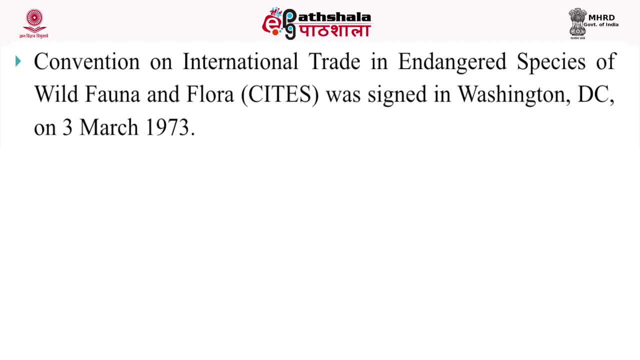 which was signed in Washington DC on 3rd March 1973.. The basic objective of this convention was there should be a complete ban that should be put on conservation of biodiversity, On trading of wildlife. the parable of the convention stated that recognition has to be given to the wild fauna and fauna in their many beautiful and varied forms. 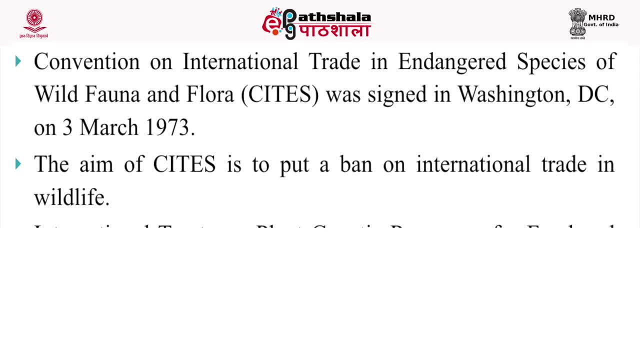 which are irrepressible part of natural system of the earth, which must be protected for this and the generations to come. Further, there is ever growing value of wild fauna and fauna from aesthetic, scientific, cultural and recreational and even economic points of view. 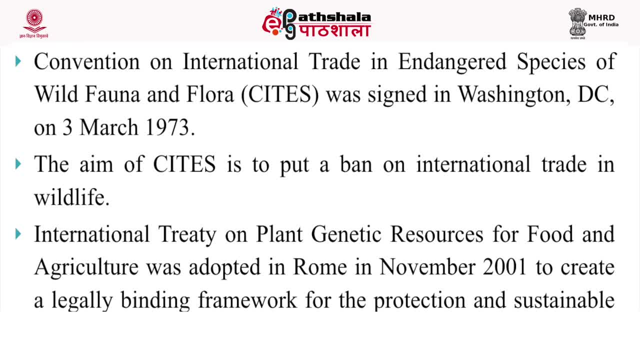 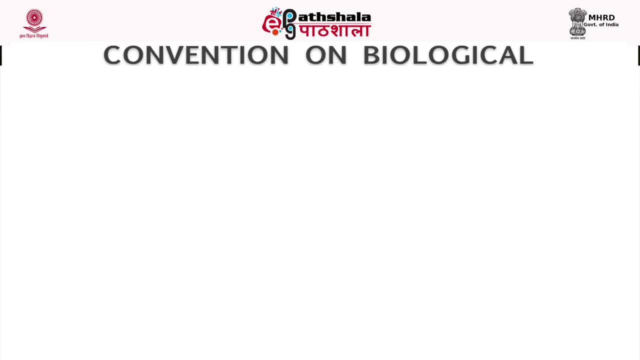 And the people and the states are, and should be, best protectors of their own wild fauna and fauna And, in addition, that international cooperation is essential for the protection of certain species of wild fauna and fauna against over-exploitation through international trade. Now the next part that we would be discussing is the Convention on Biological Diversity. 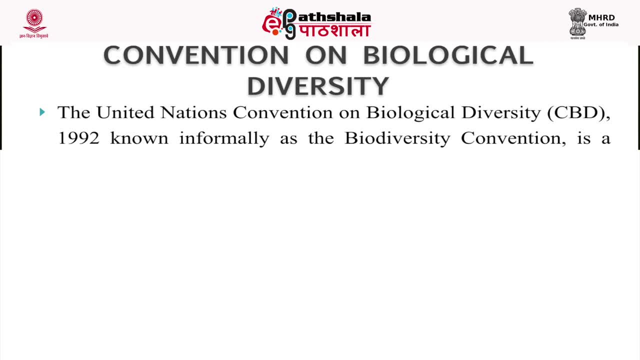 Now, the United Nations Convention on Biological Diversity, as known by the name of CBD 1992, informally also known as Biodiversity, is a multilateral treaty. This was signed in the year 1992.. The convention has three main goals. 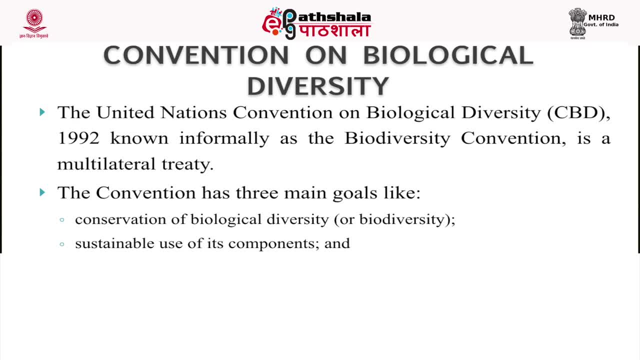 First, conservation of biological diversity. Second, sustainable use of its component. And third, fair and equitable sharing of benefits arising from genetic resources. The convention is a landmark piece in the international community and acknowledges these steps that should be taken up by the member states. 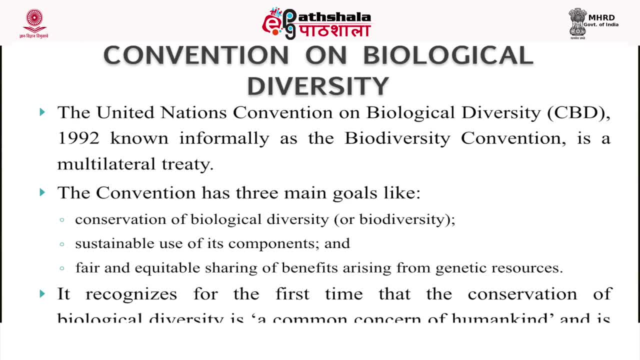 in the protection and conservation of biodiversity. It is all inclusive convention which deals with the issues, which recognizes that the conservation of biodiversity is a matter of concern for everyone, That is to say that the conservation of biological diversity is a common concern of humankind. 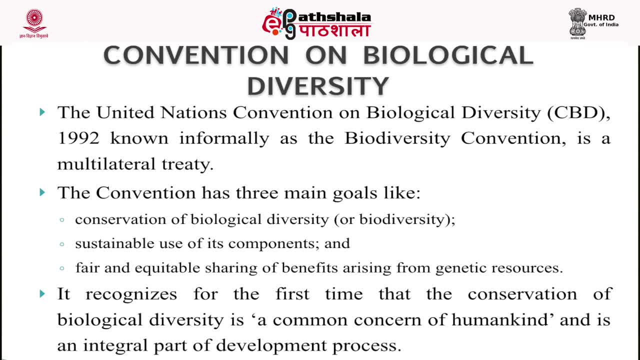 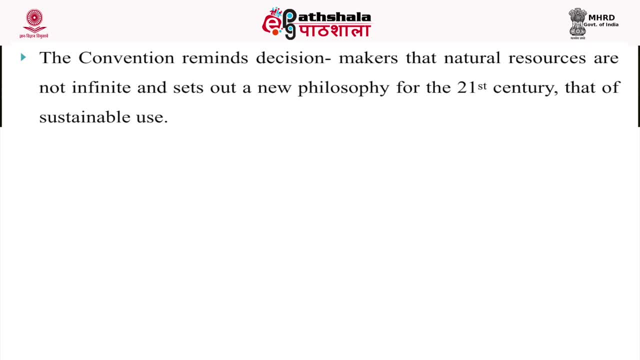 As has been pointed out earlier as well, that the resources are depleting, animals going extinct, so the international community should take immediate measures and steps for the protection of biodiversity. Some of the issues dealt under the convention are: First, measures and incentives for the conservation and sustainable use of biological diversity. 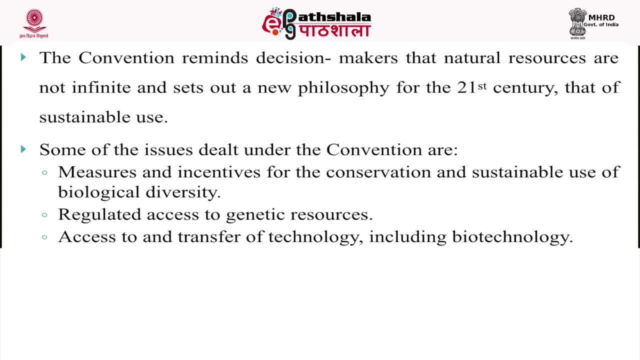 Second, regulated access to the genetic resources. Third, access to and transfer of biotechnology, including biotechnology. Fourth, technical and scientific cooperation. Fifth, impact assessment. Sixth, education and public awareness. Seventh, provision of financial resources. And eighth, national reporting. 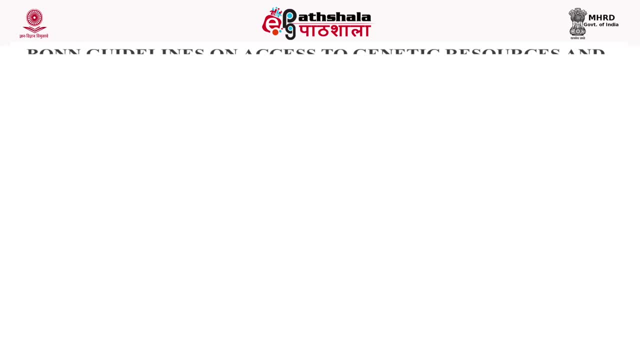 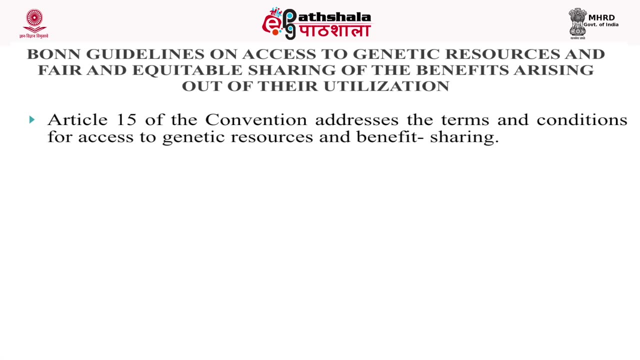 on efforts to implement treaty. The next part is bond guidelines on access to genetic resources and fair and equitable sharing of the benefits arising out of their utilization. Now, according to Article 15 of the CBT Convention, it addresses the terms and the conditions for the access to genetic resources and benefit sharing. 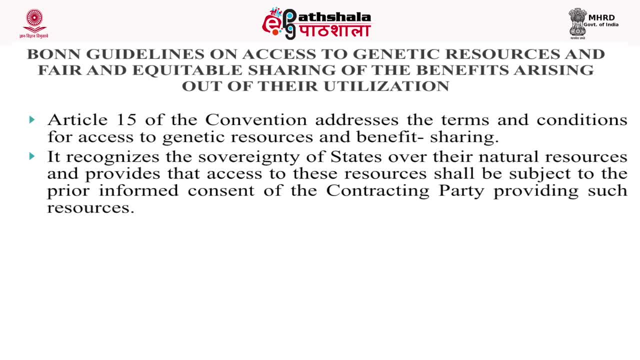 It recognizes the sovereignty of state over their natural resources and provides that access to these natural resources shall be subject to prior informed consent of the contracting parties providing such resources. So, therefore, in consonance to this article, these guidelines, that is, the bond guidelines, 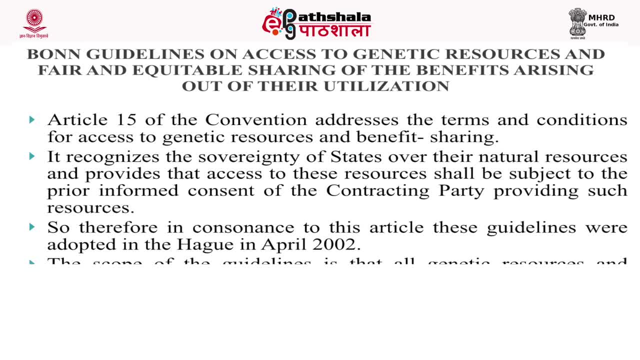 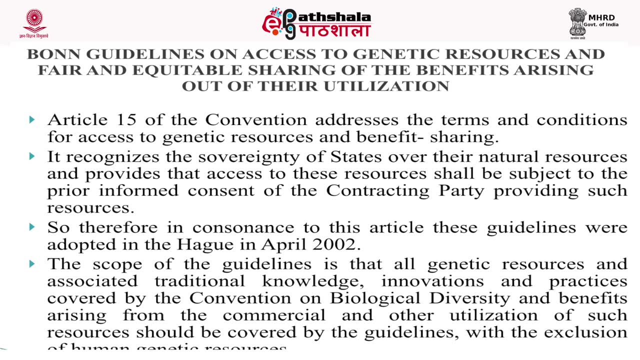 were adopted in The Hague in 2002, April. The scope of these guidelines is that all genetic resources and associated traditional knowledge, innovations and practices covered by the Convention on Biological Diversity, and benefits arising from the commercial and other utilization of such resources should be covered by the guidelines. 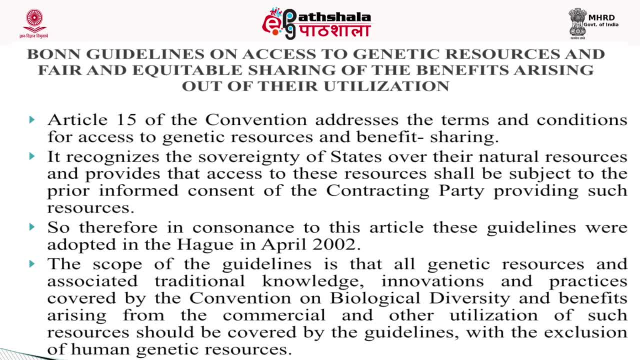 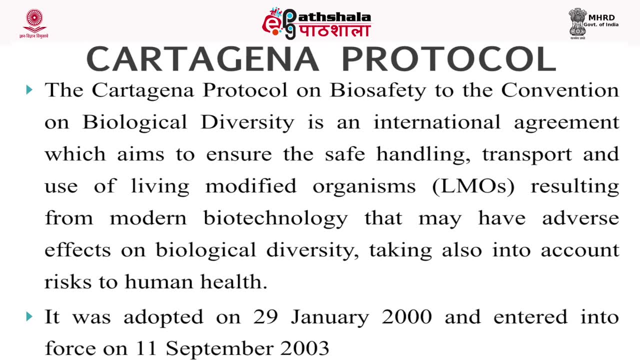 with the exclusion of human genetic resources. One of the objectives of these guidelines, in addition to the other, is to contribute to the conservation and sustainable use of biological diversity. Now the next part is the Cartegna Protocol, The Cartegna Protocol on Biosafety to the Convention on Biological Diversity. 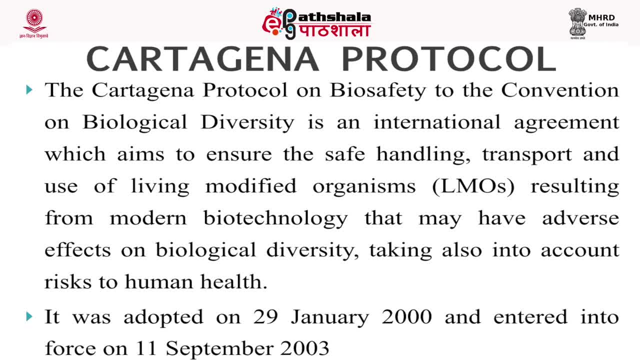 came into force on 11th September 2003.. with the basic goal to ensure the safe handling, transport and use of living modified organisms resulting from modern biotechnology that may have adverse effect on biological diversity, taking also into account the risks to the human health. 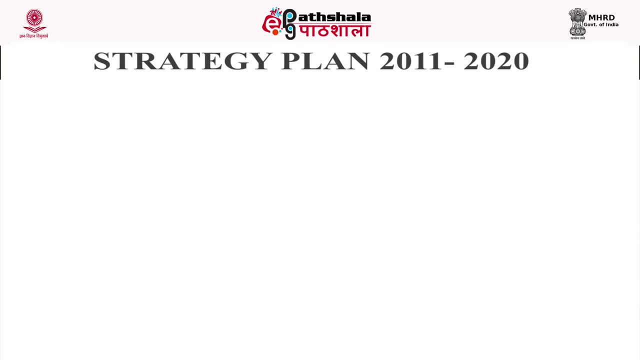 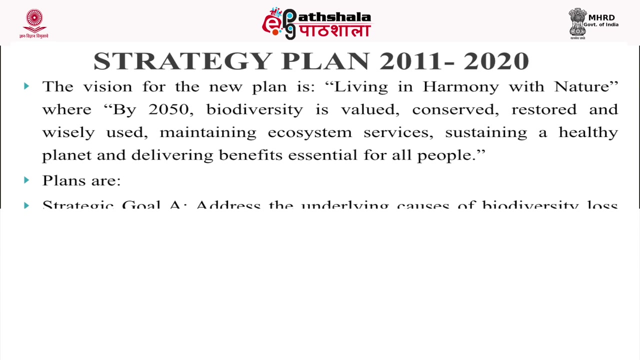 Now, the next effort which was taken by the United Nations was the Strategy Plan 2011-2020.. The rationale for the new plan is that biological diversity underpins ecosystem functioning and the provision of ecosystem services essential for human wellbeing. It provides for food security, human health. 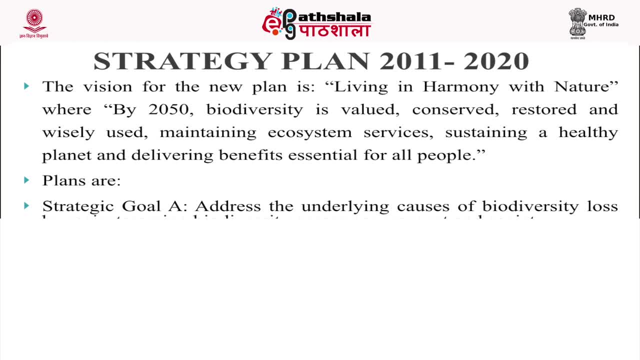 the provision of clean air and water. it contributes to local livelihoods and economic development and is essential for the achievement of millennium development goals, including poverty reduction. The vision of the new plan is living in harmony with nature where, by 2050, biodiversity is valued. 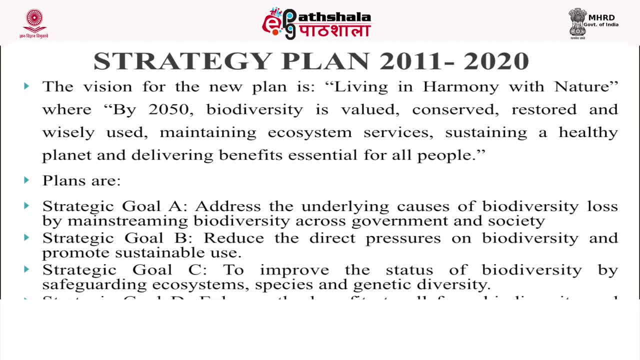 conserved, restored and wisely used, maintaining ecosystem services, sustaining a healthy planet and delivering benefits essential for all people. The mission of the new plan is to take effective and urgent action to halt the loss of biodiversity in order to ensure that by 2020, ecosystem are resilient. 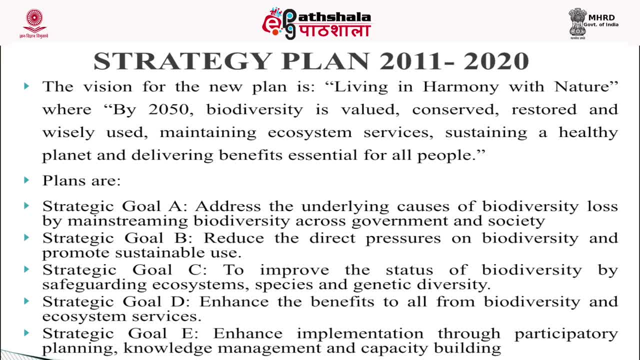 and contribute to provide essential services, thereby securing the planet's variety of life and contributing to human wellbeing and poverty reduction. To ensure this, first, pressures on biodiversity are to be reduced. second, ecosystems are to be resorted. third, biological resources are sustainably used. 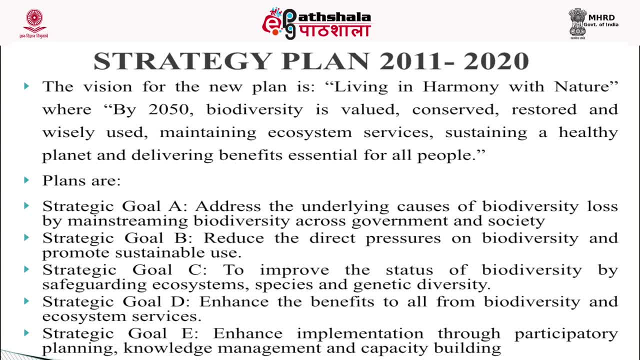 and last, benefit arising out of utilization of genetic resources are shared in fair and equitable ways. The strategy plan consists of 5 calculated goals and includes 20 biodiversity targets. The strategies are First: Goal A Addresses the underlying cause of biodiversity loss by mainstreaming biodiversity across the government and society. 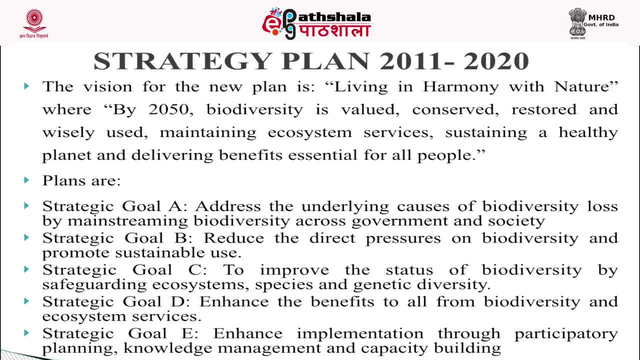 Goal B: Reduce the direct pressures on biodiversity and promote sustainable use. Goal C: To improve the status of biodiversity by safeguarding the ecosystem species and genetic diversity. Goal D: Enhance the benefit to all from biodiversity and ecosystem services. Goal E: Enhances the implementation through participatory planning. 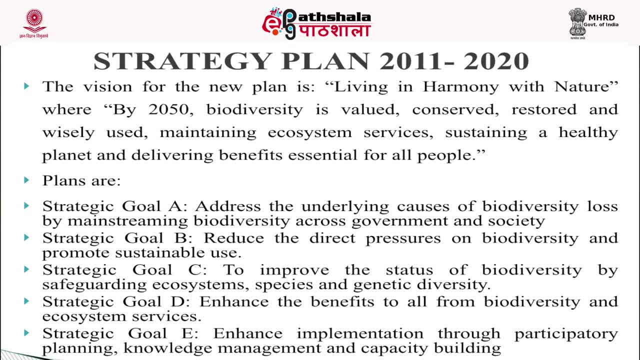 knowledge management and capacity building. The next part is Conservation of Biodiversity and India. India has been taking various steps for the conservation and protection of biodiversity, and one of the pertinent step in this direction was becoming a part of the Convention of Biodiversity. 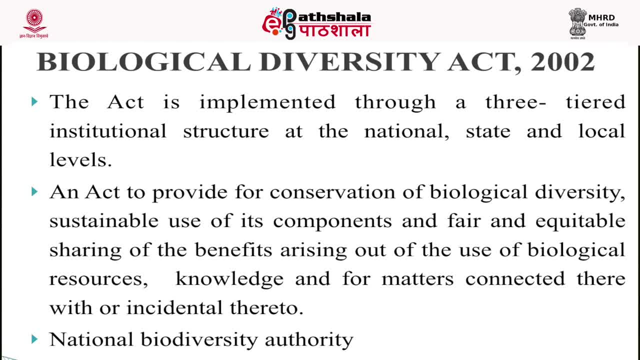 In consonance to this, India made a law called the Biological Diversity Act 2002.. India made a law for the protection of this. as I have already discussed that, the name of the act is Biological Diversity Act 2002 and notified the rules called as the Biological Diversity Rules 2004. 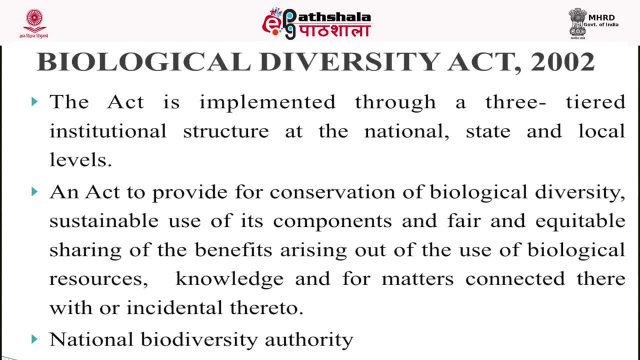 in consonance with the CBD, India became a party to the Convention and brought it into force on May 19, 1994.. The preamble of the act states that it is an act to provide for the conservation of biodiversity, sustainable use of the components. 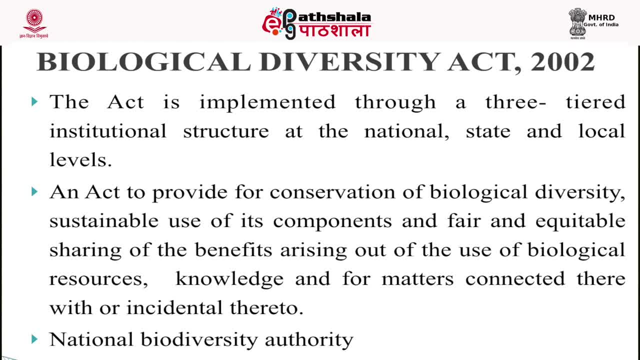 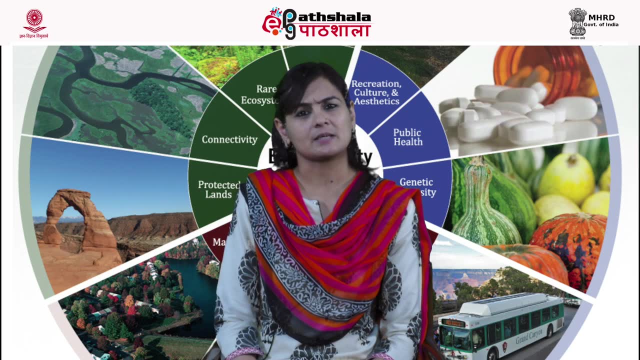 and fair and equitable sharing of the benefits arising out of the use of biological resources, knowledge and for matters connected thereto and incidental thereof. Now, as my topic of discussion was conservation of biodiversity, we have basically discussed: what was the definition of biodiversity, what exactly is the importance of biodiversity? 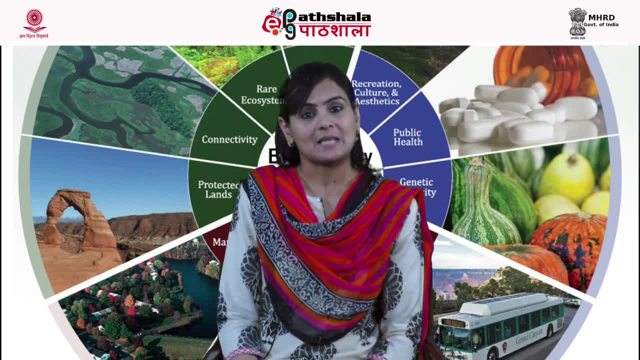 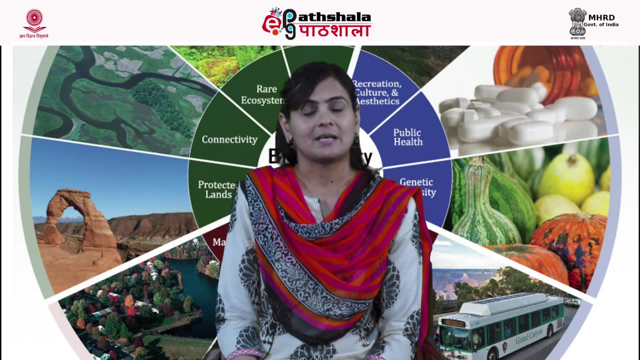 what are the reasons for the loss of biodiversity and what steps have been taken by the United Nations for the preservation and protection of biodiversity? Now we need to end this by stating the fact that nature has been very kind to the human being, but at the same time, it becomes the duty. 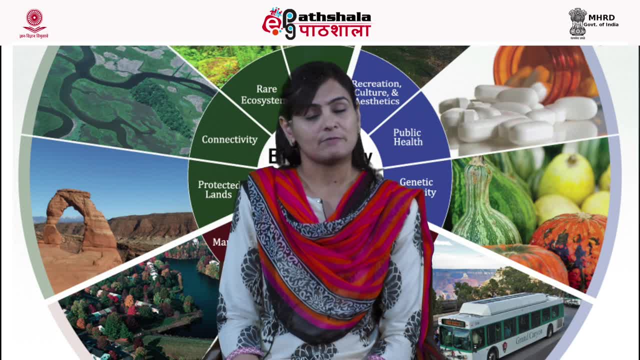 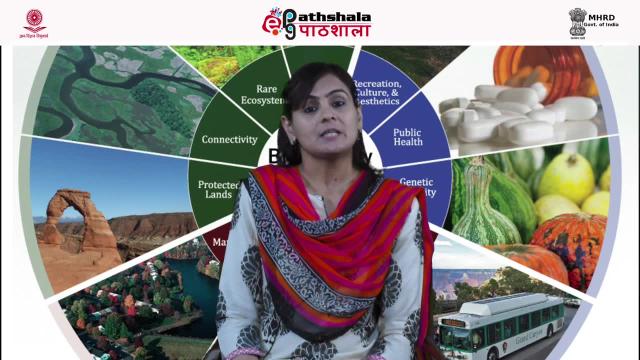 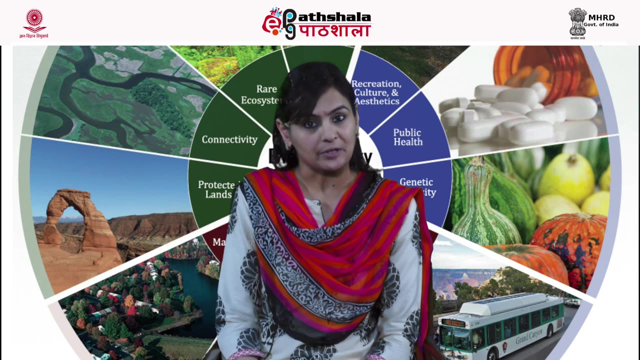 it becomes the obligation of the individual to take every possible effort for the conservation and protection of biodiversity, and we further need to recognize this, that we need to accept the fact of sustainable development, wherein we are not just preserving our resources, our biodiversity, for present, but also to keep in view or in mind the future needs as well. 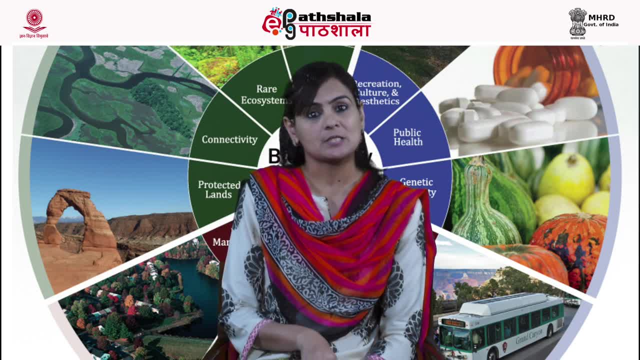 Therefore, as India has taken a very important step by passing of this act, every possible effort should be made for the conservation and the protection of biodiversity. Thank you.